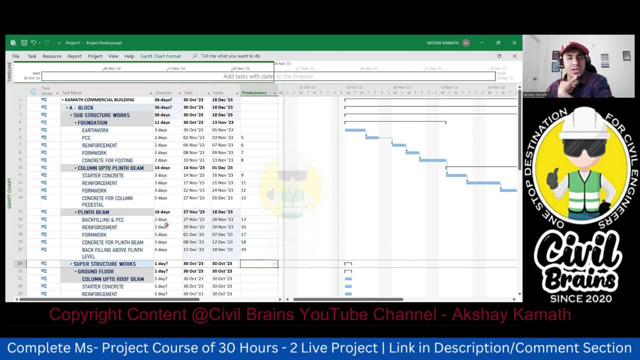 there was a uh question mark coming. the reason was that here i had not given any days right, so that so in the substructure part foundation column up to plinth beam and plinth beam was dead. so from earthwork to this, everywhere the duration is given. so how many, totally, how many days is? 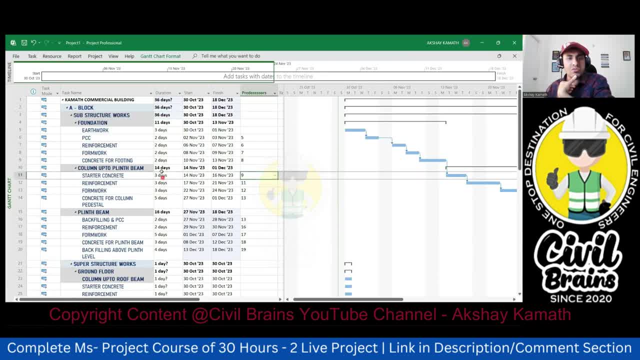 required 36 days. how did i come to know? 11 plus 14 comes out to be 25. 25 plus 16: 35. how much it is so? 11 so 14 plus 11 is 25, right? yeah, 25 so 35, it should be 41. no, then why it's not coming? 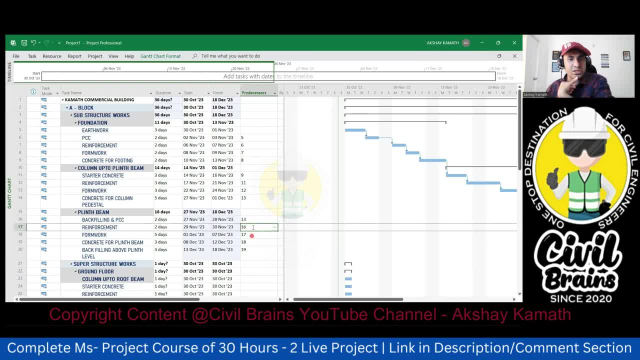 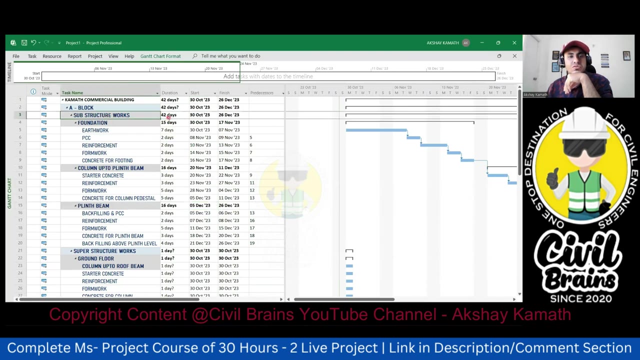 maybe some, some links, some link. we are not connected. i feel that is why it's not showing. earthwork should have come now. wait, yeah, so i given the activities, so this is fine. i think this particular thing, the substructure, were 42 days. it's not reflecting, i don't know why. let me check it out in the next lecture and 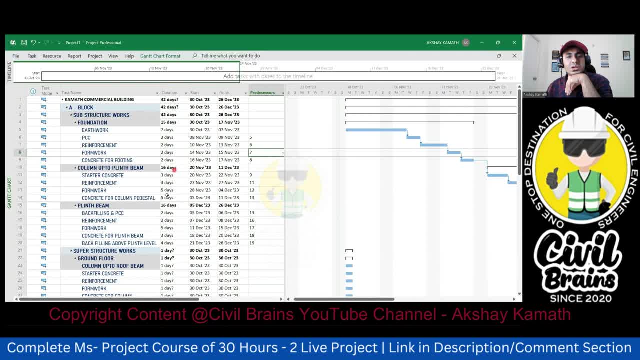 i'll update you, because 15 plus section is 31. 31 plus 16 should come out to be 40, 46, 46, 47 days, but it's coming only 42 days, so i don't know why it's coming like that. we'll check. 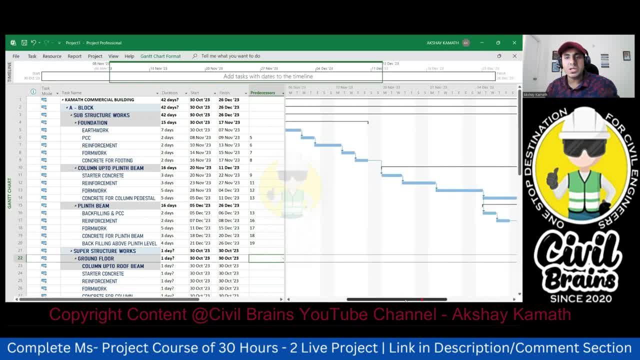 that in the later, but not an issue. okay, anyhow, now you come to the right side. okay, now try to understand this entire concept. so what i'll do see right now if i come here. okay, it's not looking good. no, i mean, few of my activities are coming here. half of the activities are going the right. 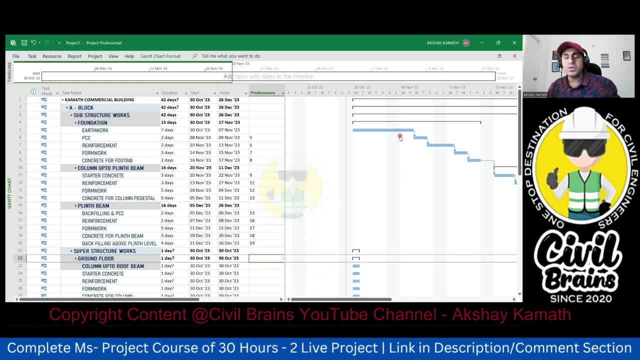 side. so i want all this gan chart to be seen in one particular shot. so what i'll do? i'll: right click here, go to the option. so right click here, go to the option called as zoom. okay, you have to keep your mouse here. right click, go to the option called zoom. here go to the option called as entire. 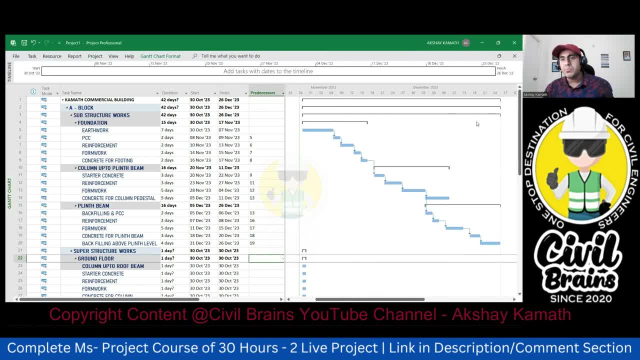 project and say, okay, so now you can see entire project, you can see it here, got it now. what is these things? so you need to understand all these things. so this is the start of the project, this is start and this is the end portion. okay, start and end. so 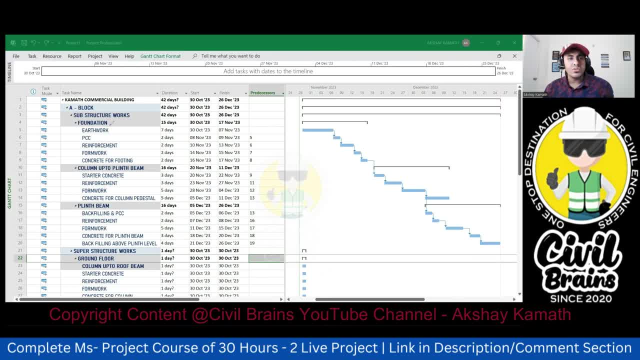 yeah, fine. so now you see here this kamath commercial building. so under the kamath commercial building, all the things are coming, isn't it? from start to the end, up to third floor, from a block to the third floor, last de-shuttering, all the things are coming under kamath commercial. 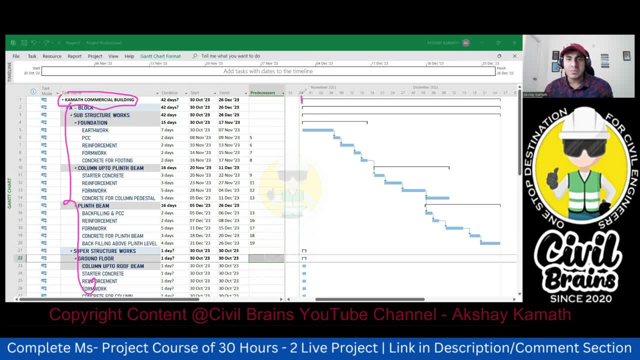 building. so the same thing you can see here. so this is the start of the kamath commercial building. this is the end of that. okay, under this, only under this, you can see all these activities is under this. this is the last line. under this, only all the activities are coming right. so how? 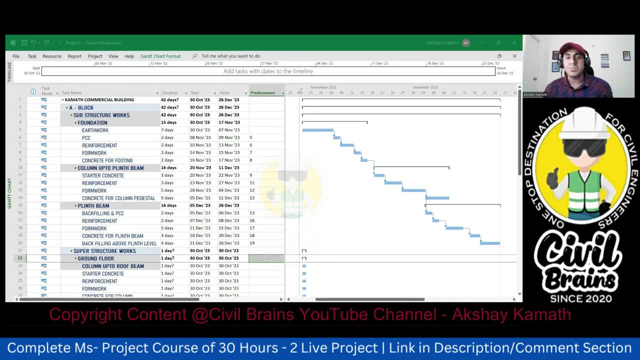 did it come because that is what we had given work breakdown structure. so this is called a summary task. i will write it here. it's called as a summary task. got it? yeah, good, now, after that. next is: what a block? so this a block? you see, here it is starting from here. this is your a block. this. 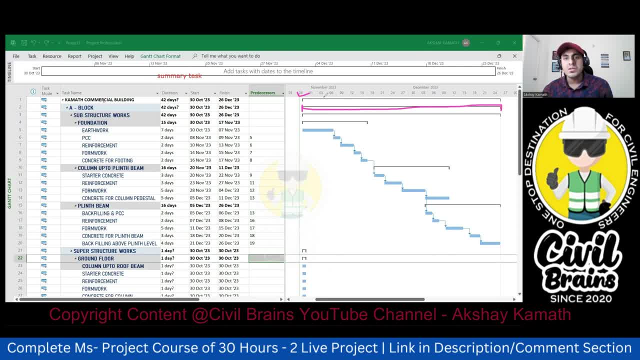 also will go up to here. so this a block is coming under kamath commercial building. so this is kamath commercial building. the second line is your a block. now come to the third point. what is that? substructure work. now again, substructure work also will start from this date. it will go to this date. 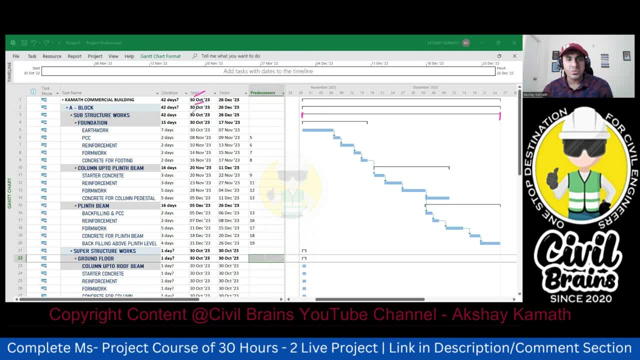 okay, see the date: 30 october, 30 october, 30 october, end is 26, 26, 26, so 30, 30, 30, end is 26, so that is why all the things are in the same line. only the thing is, this is your kamath commercial building. 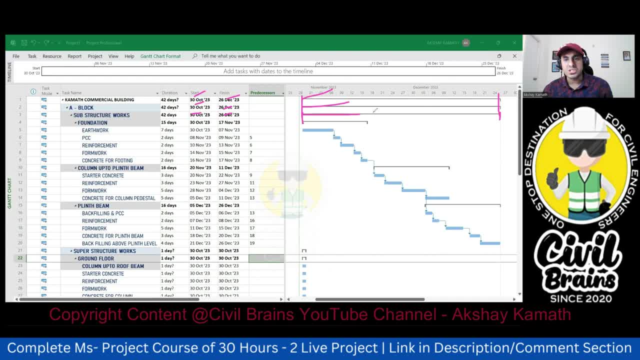 line, this is your, a block under that your substructure, substructure work will come understood. you now come to the third, fourth point: foundation. the foundation. it is starting from 30 october and it will go on till 17th november. so this is your: 30 october, this line and this is your. this is. 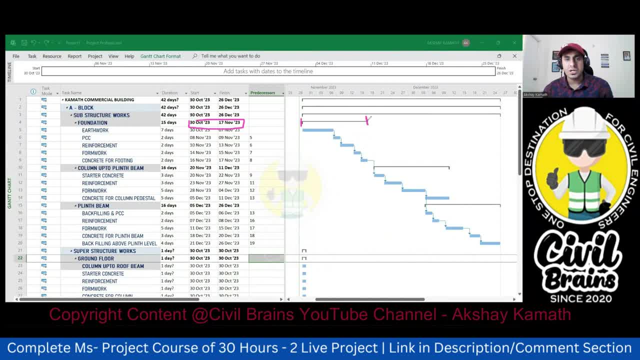 15, isn't it? so this is your 17th november line. got it, got it simple. now, under the foundation, what all is happening? earthwork is happening, pcc is happening, reinforcement, form work and concreting. so this is your earthwork. okay then, this is your pcc, this is your reinforcement, this 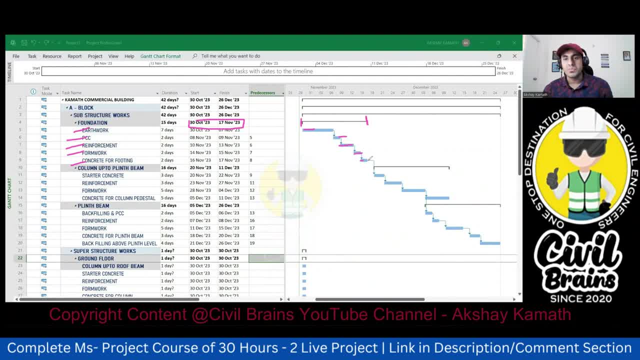 is your form work and this is your concreting work, isn't this? isn't that all these things are falling under? so it's starting like this and this is the end of that summary task. so all the activities are coming under this, isn't it earthwork? then we have pcc, we have reinforcement, we have form. 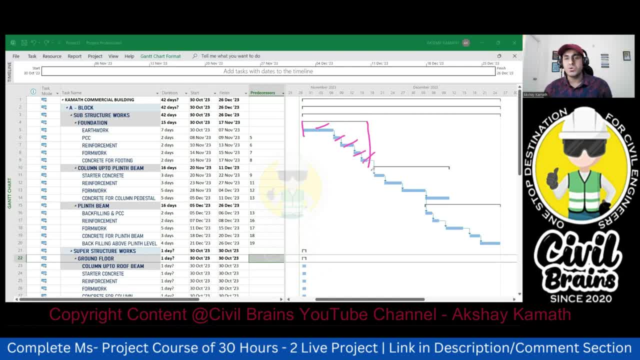 work. we have concrete per footing. understand how it's going, how you are going to read it again. by looking at this you can understand everything is finished. to start that means only after this activity, that is, which activity- earthwork- is finished. we'll start with the pcc only after. 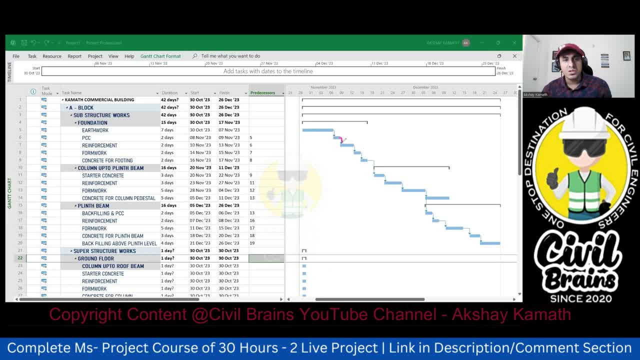 the pcc is finished. only after the pcc is finished we'll start with the reinforcement. only after the reinforcement is finished we'll start with the formwork. only after the formwork is finished we'll start with the concrete for footing understood the concept. so this is how the 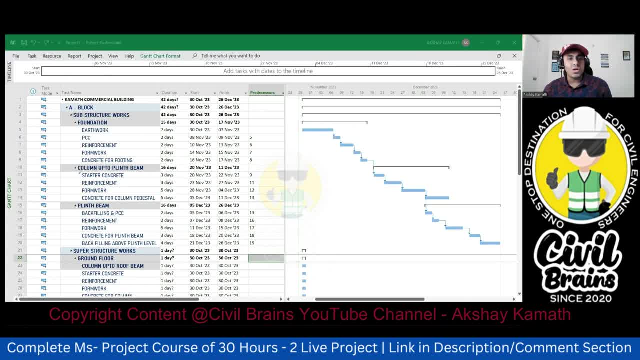 interlinking is done after that. next is what? column up to plinth beam. again, this is a summary task. so this is your column up to plinth beam, which will start from here. it will go up to here. so why it is starting from here? because the date is 20 november, so 20 november will be somewhere. 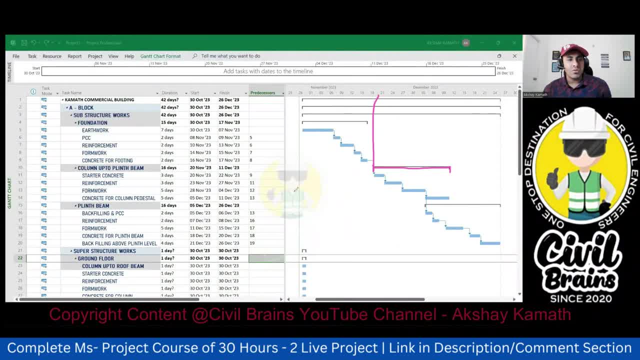 here, here, like this: okay, this one understood now under the column up to plinth beam what all things are coming. starter concrete: so this is your starter concrete, this one small portion, then reinforcement: this is your reinforcement. then take one minute. so starter concrete: yeah, this is your starter. 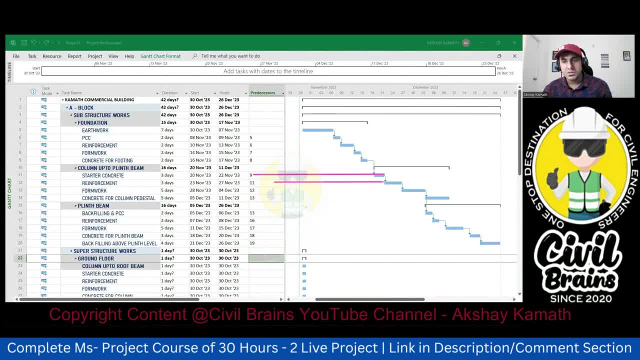 concrete. this is your starter concrete. yeah, this is your starter concrete. yeah, this is your concrete. then this is your reinforcement work. this is your reinforcement work. then, after that, this is your formwork, and the last one is: which one concrete up to pedestal this one? so, from 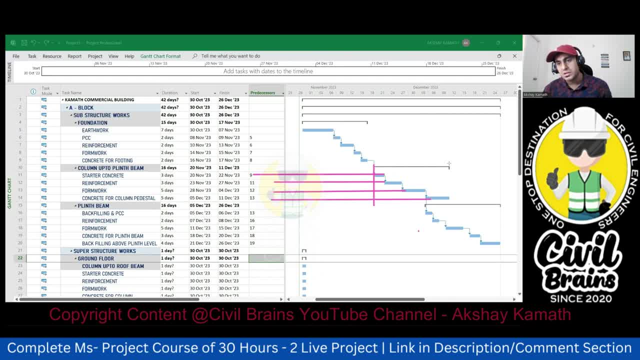 inside this, only all things are happening from this side to inside. this is a summary task. right, understood the concept. so in this way you can uh visualize, you can check your uh, this thing bar chart here. so all the activities will fall in between to this activity. so wherever you get, 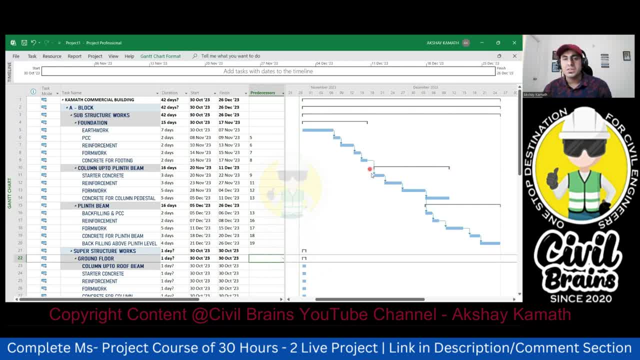 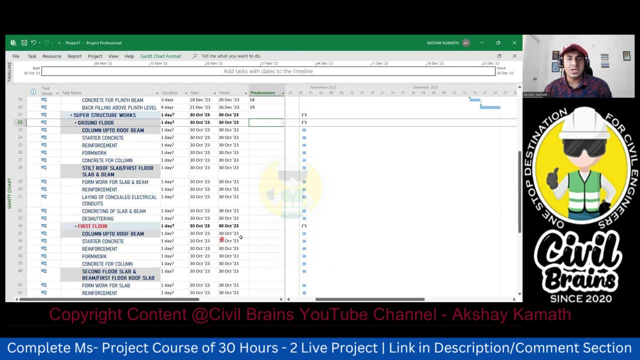 this straight line, isn't it like this? so this line is called as a summary task. what it? so? this particular line, whatever you have, it's called as a summary task. understood the concept here? i did not do the interlinking, so that is why it's showing like 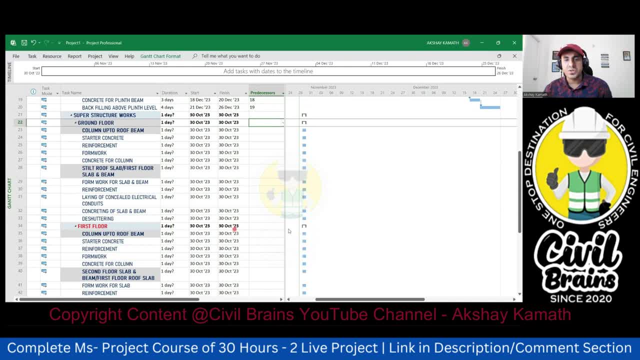 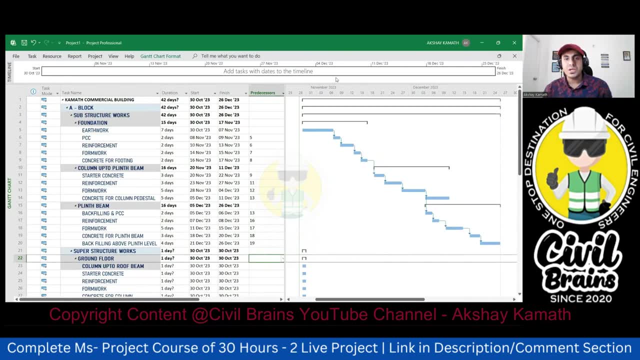 this. but wherever there is a summary task, like first word, this is a summary. you can see, this is a summary task is created here. understood the entire logic. good now, if i right click here, if i right click here and if i go to the time scale- not this one- if i right click here and if i go to the bar style previously. 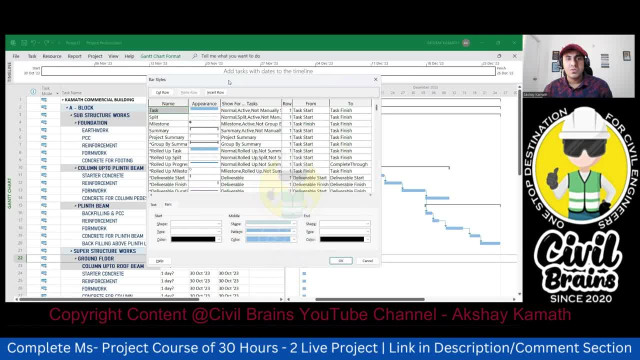 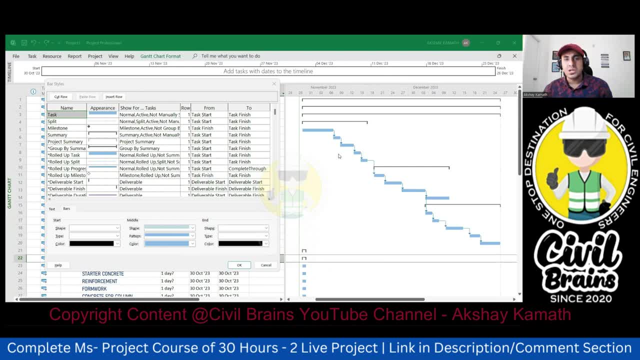 i had told you one thing that previously, what did i tell? i told you, told you only about the task option, isn't it? later, we did not speak about the split milestone and all now we have this. this is called a summary task. we can see here summary. 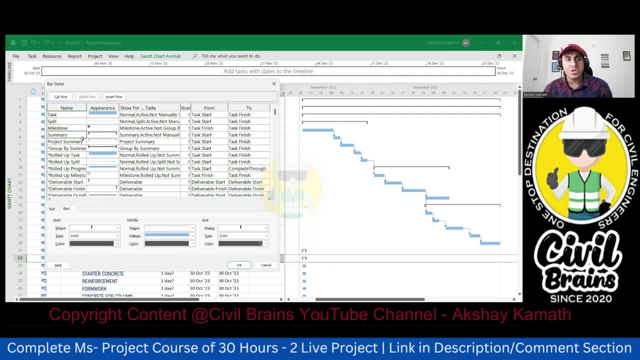 and you can see this particular pattern. the same pattern is followed here. got it? so this is summary. now click on the summary. come to the this thing. what is that? how to change it? yeah, come to the summary. now you come to this one. if you want to change the shape of this, you can change it now, so i'll keep it. 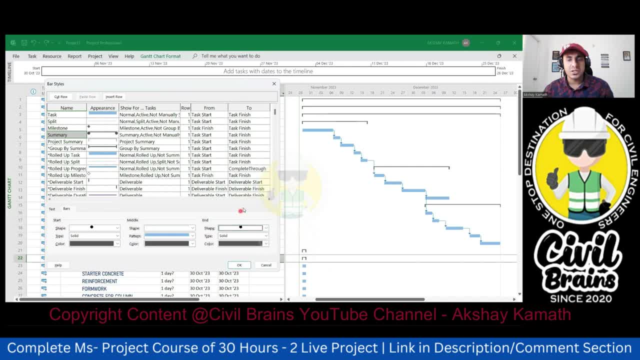 like this end also. i'll keep it like this, got it. and middle, middle, let it be like this, only not an issue color. if you want to change, i'll say: uh, color. you give red color to the start, you give red color to the end and middle portion will make it little green in color. okay. 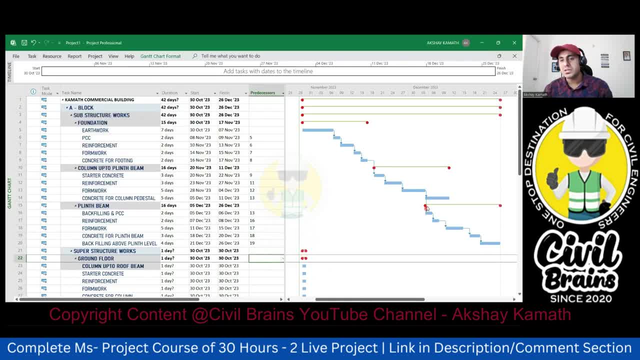 and i'll say: okay. so can you see this now? summary task. what happened? i went and changed the summary task from there. now you understood the concept, okay. so whatever lines, you can see it now here: if i right click, go to bars- time and then, if i click on 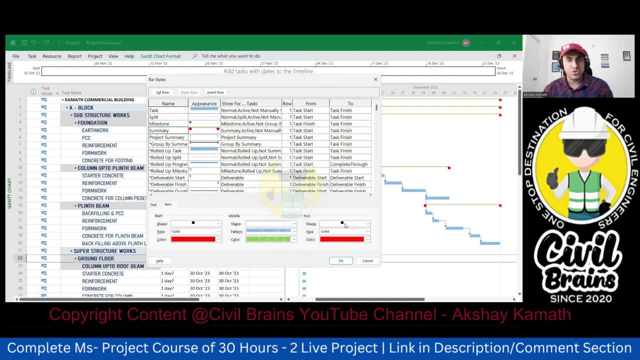 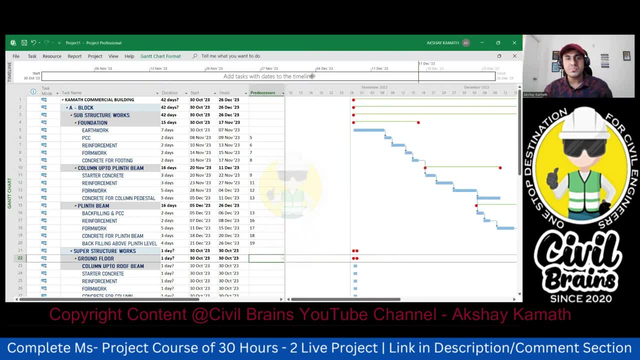 summary and you can see. this is the pattern, what i've given. if you don't want, come here change everything from here. understood the concept? good, now we'll come to the last concept here. so the last concept is about the level. go to the task. i hope at least this much understanding is done. go to the task option. 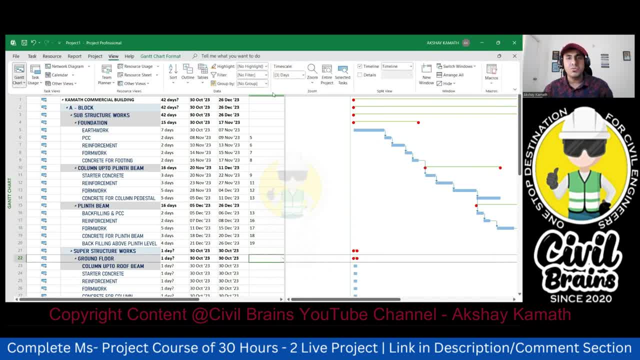 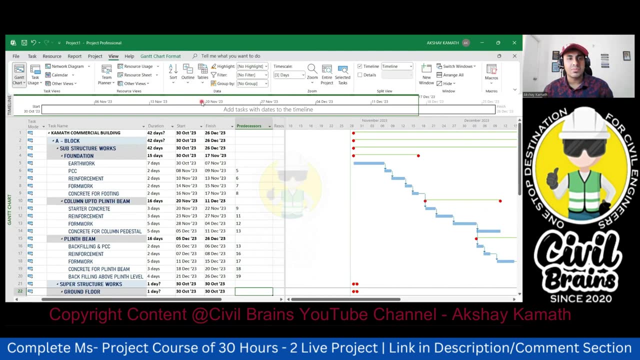 this option, not task. go to the view option. so in the view there is option called as: yeah, go to the view option. in the view there is option called as outline. click on the outline. so here show subtask, not this one. height subtask. okay, all tasks. okay, go to level one. 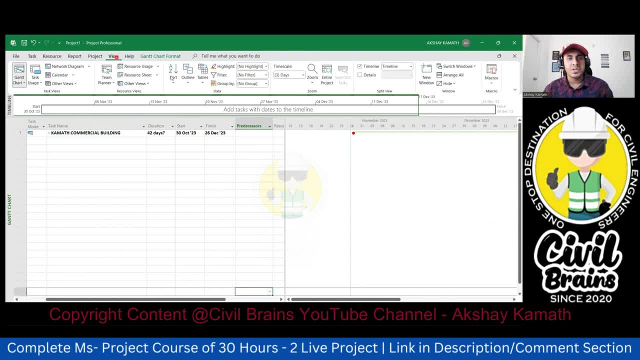 see. so what you are supposed to do: go to the view option in the view, go to the outline option, go to the level one. so this is the level one schedule. that means kamath commercial building. this is level one. somebody asked you, akshay, show me the. 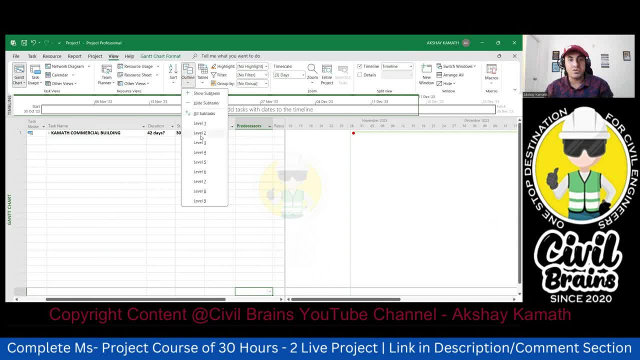 level two task. so level two. so come here, go to level two. so what happened under the common commercial building? there was a, a block, suppose. if there was b block also then, and if i had given a b block, then even b block would have come on inside this simple. now tell me what is level three schedule. 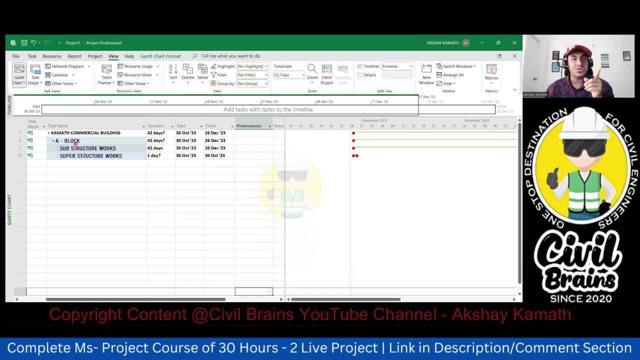 you have level three. in the a block we had substructure work and we had so per structure work. good, this is level three. come to level four. so, and exactly under the substructure, we had foundation, we had column up to print beam, we had clean beam. in the superstructure work we had ground floor, we had first floor, we 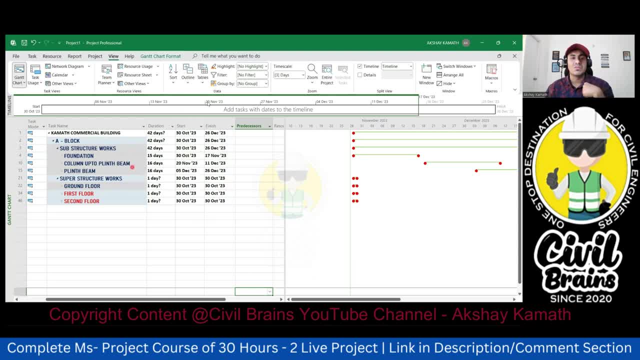 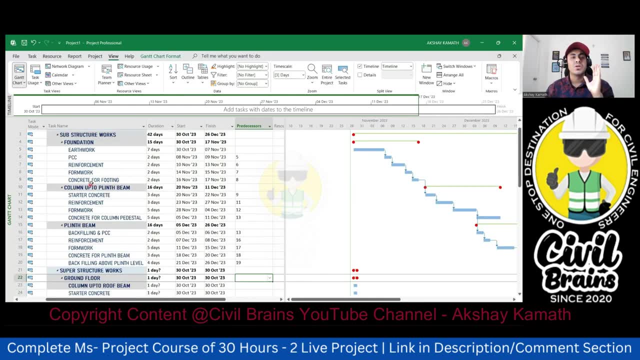 had second floor. show me the level four schedule. so this is level four. show me the level five schedule. good, under the foundation we had earthwork, pcc reinforcement formwork, concrete. then under the column up to plane beam we had starter concrete reinforcement formwork, plinth beam. we had this one then. 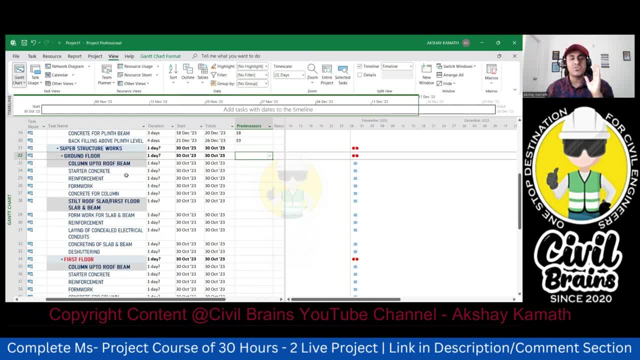 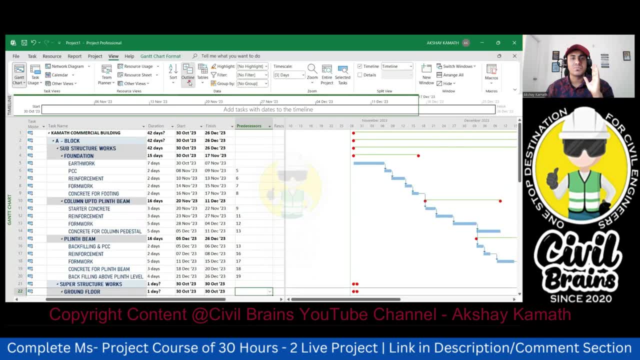 under the ground floor we had column up to roof beam starter concrete reinforcement and then first floor, we had this one. second floor, we had this one. understood, so this is called as level. okay, now up to which level we finished level five. i finished. now, if i click on level six, there's no. 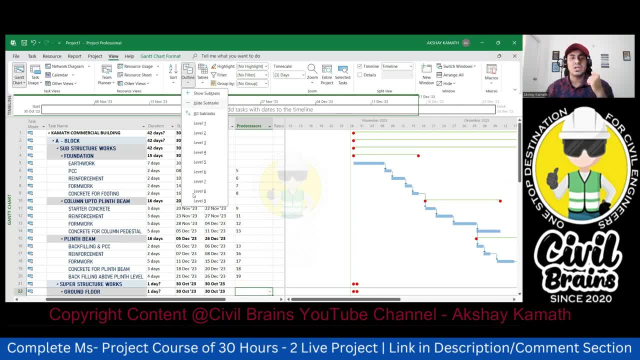 change. if i click on level seven, there's no change. if i click on level eight, there's no change. so what do you mean by this? that means my work breakdown structure. whatever i had done, i i did up to level five right, or level four, level five. so my work breakdown structure, whatever i had. 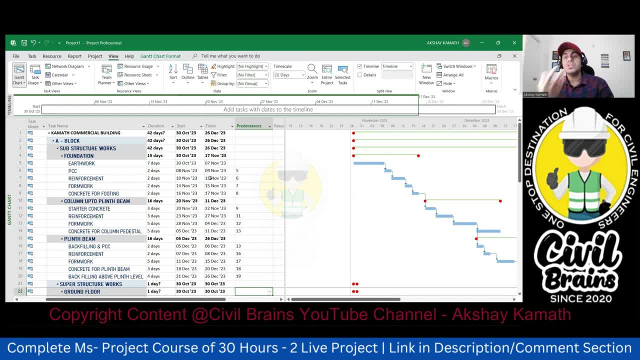 done. it was a level five schedule, level five breakdown what i had. further, if you want to do, you can do it. i'll show that in the next lecture how it has to be done. so now understand the concept. okay, your boss told you: uh, show me a preparer level two schedule. so what is that? 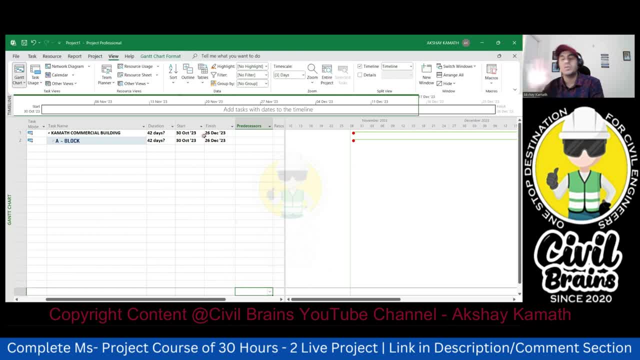 level two schedule. this is a level two schedule. kamath commercial building a block. your boss told you prepare a level three schedule, click on level three. so in the next lecture i'll show you how to prepare a level three schedule. click on level a block. we have substructure and superstructure. then somebody told you your boss told, go and do. 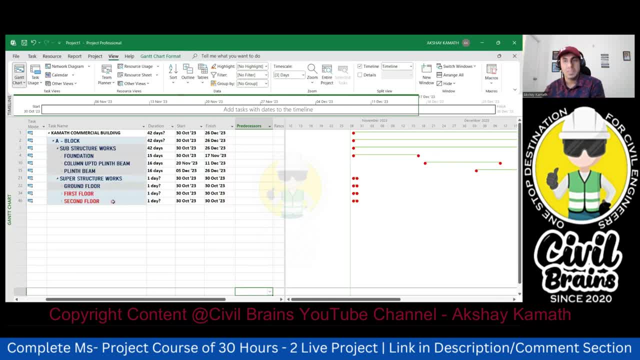 me, show me a level four schedule. so this is level four schedule. understood the concept. so this is like a bird eye view. that is kamath commercial building is a bird eye view. finish, just you're seeing from the top. now if you want to go inside that, come to the level two- a block. then if you 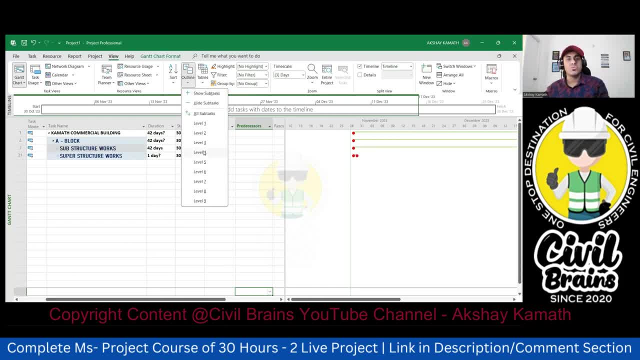 want to go even more into that, come to the level three. even if you want to go more into that, level four. got it. so this is how you are supposed to understand it. now there are two things which you need to understand. uh, one is- uh, yeah, one is micro level. 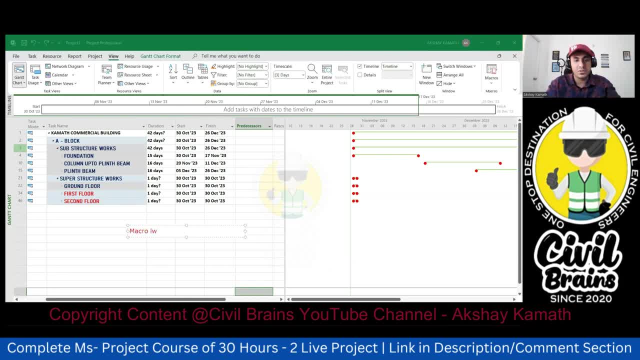 one is called as macro level, macro level. the second is called as micro level, micro level. so this macro level is a higher one, your level, one level one is a macro level, which i say, which is less okay, which is a less level, and micro level is the last level, last level, last level. so here in the ms project, the last level is: 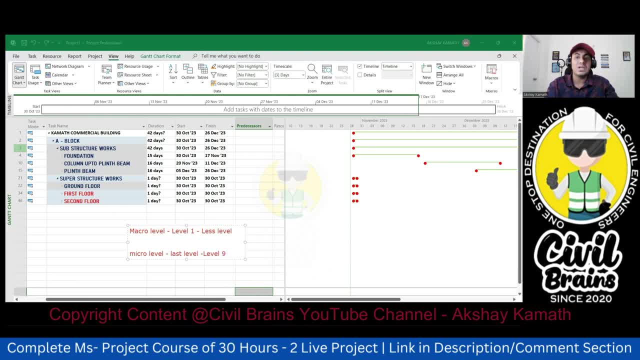 level nine, isn't it level nine? but it depends on what level you are creating in your project or whatever building you are taking. uh, if level five you have, if you have done a level five schedule, then level five is the last level for you, which is a micro level, but in the ms project, by default only. 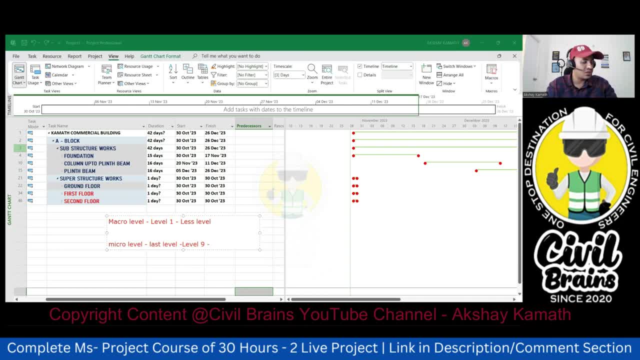 level 9 is available and this is called as the which level. if it is less level, this is more level. okay, more level. or you can call this as more detailing, more detailing, and here it is less level, or you can call this as a less detailing, you can. 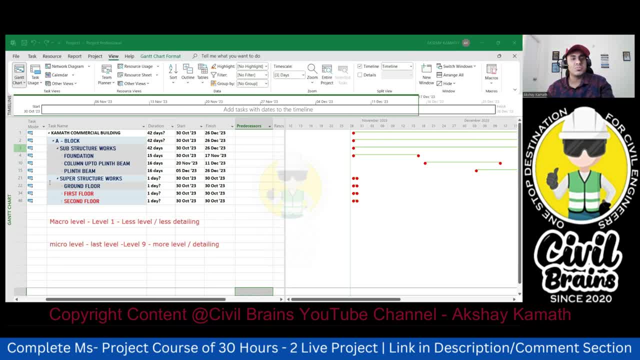 note it on all these things. yeah, understood the concept. yeah, so micro level means you're going in depth and macro level means from the top you are seeing. in the macro level it's like a first level, second level, so the lead, the detailing, is very less. in the micro level you'll be in the last. 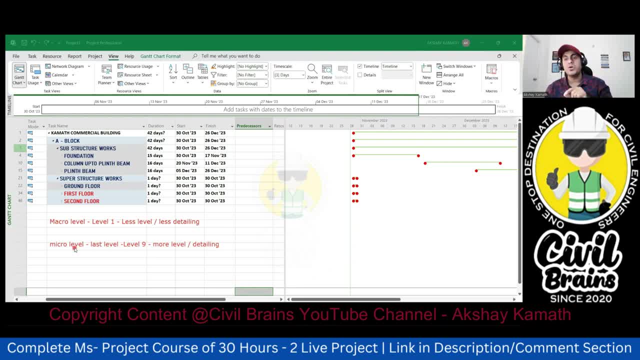 level. so in the ms project the last level is level 9. but if you are doing a work breakdown, it depends up to you what is a, what is a last level that you have, whether it is level 4 or level 5 and it has more level or it has more detailing. simple now understand one thing in the outline. if i go to